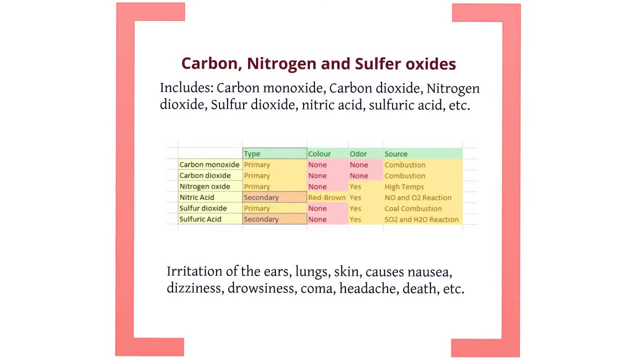 monoxide, carbon dioxide, nitrogen dioxide, sulfur dioxide, blah, blah, blah, blah blah. I couldn't find a nice chart, so I made one. This is a little chart that shows you the type of pollutant they are, whether or not they're primary or secondary, the color they have, the odor. 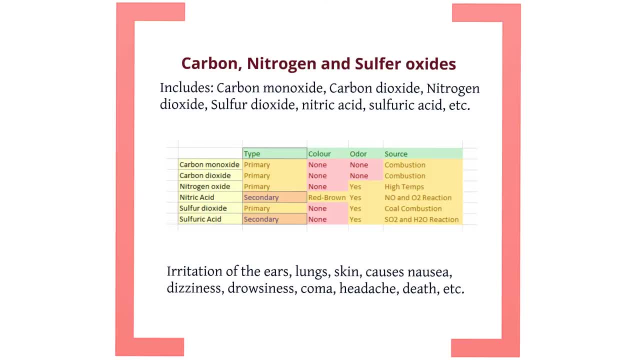 and the source. If you take a look at the sources, you'll notice that a lot of them have to do with combustion. Whenever you're burning things out, you're creating a lot of these. Also one thing to note: everything except nitric acid has no color, so it's not. 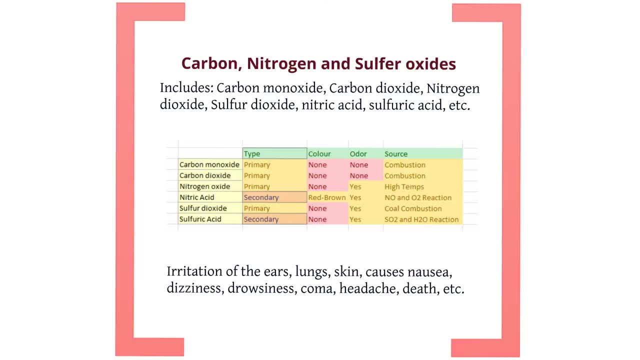 something that you can see, And carbon monoxide- carbon dioxide- don't really smell very much, though the nitrogen oxide and acid and sulfuric acid does smell. These can cause irritation of the ears, lungs, skin causes nausea, dizziness, drowsiness. 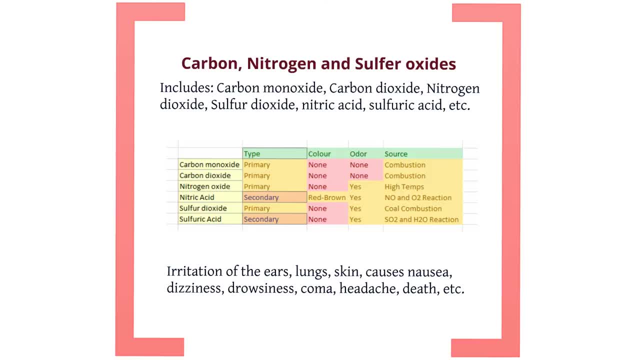 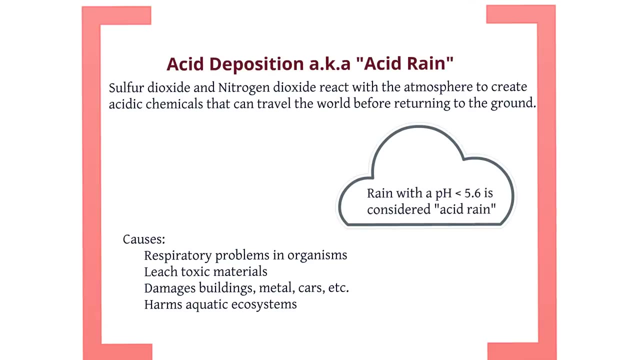 coma, headache or death. Carbon monoxide is also one of the main reasons. carbon monoxide poisoning and suffocation is one of the main reasons people die in fires, Moving on acid deposition, also known as acid rain, Sulfur dioxide and nitrogen dioxide. 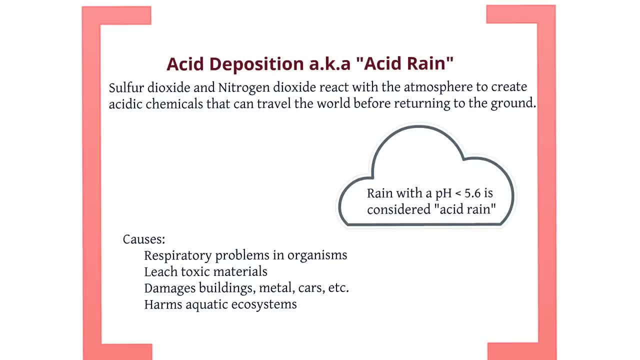 react with the atmosphere to create acidic chemicals that can travel the world before returning to the ground. Acid rain is considered to be rain with a pH of less than 5.6, and some of the problems that it causes are respiratory problems. on organisms, it can leach toxic materials if. 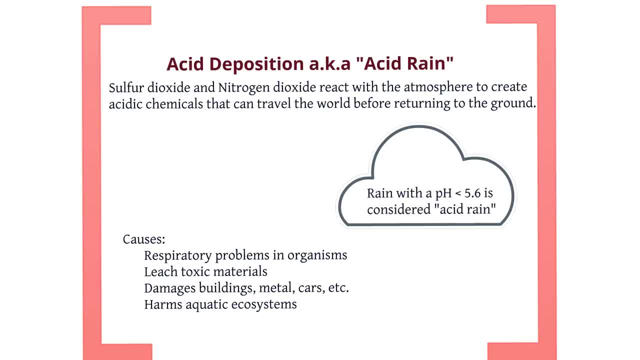 it lands on them. it can damage buildings, metals, cars, the paint job on your car if it rains, yeah, that's going to be damaged. Next it can also harm aquatic ecosystems, simply because the water will just keep piling on there. there's really no way to get it. 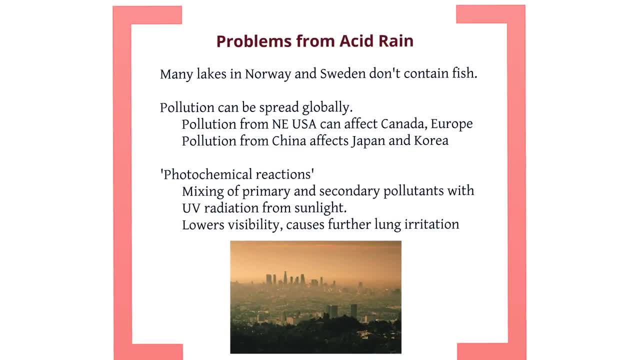 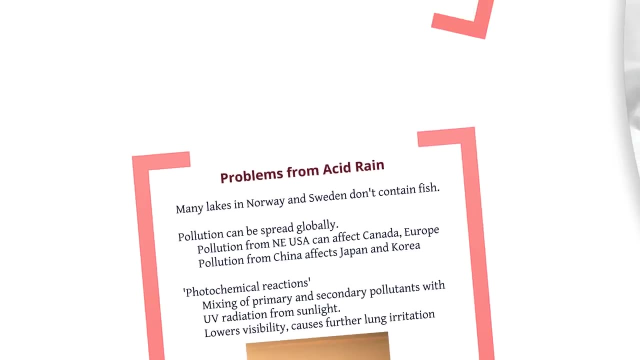 out of them. So some of the problems with acid rain. many lakes in Norway and Sweden don't contain fish because the water has become so acidic that the fish have died, Not to mention pollution can spread globally. In the previous slide, if we just go back to it, it says that they. 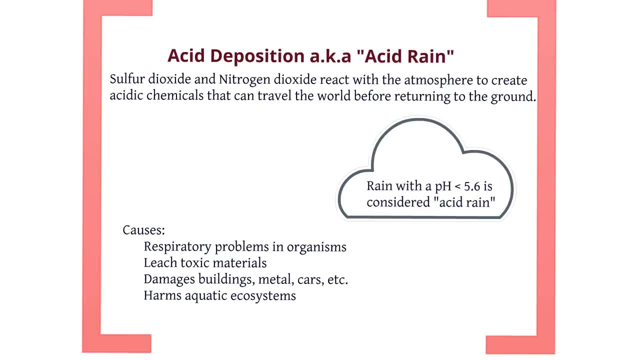 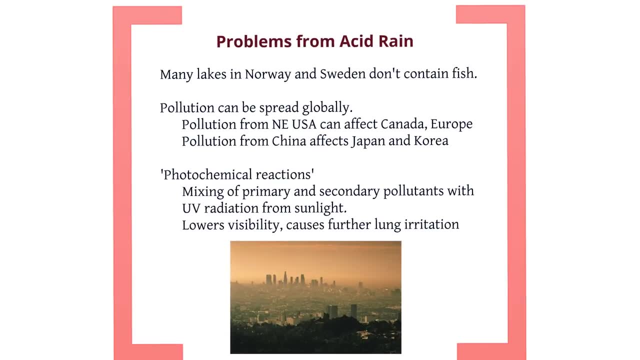 can travel across the world. just because the chemicals are floating around in a cloud doesn't mean that a cloud is going to stay over within a one mile radius of that city. That cloud can float all around the world, So it can cause some problems globally. So 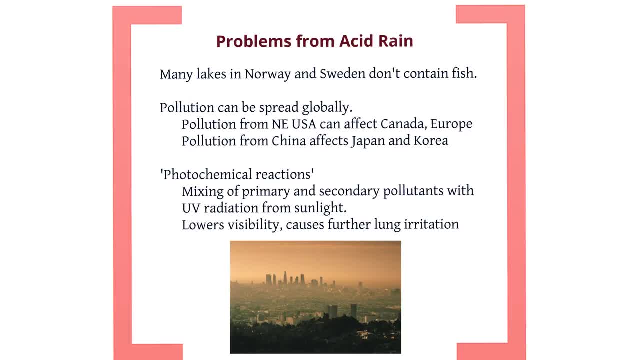 Pollution from the Northeast United States can affect Canada and Europe. Pollution from China can affect Japan and Korea. So it's not just your city that you are polluting, but it's also the entire global system that you're also affecting. There's also these things called photochemical reactions. 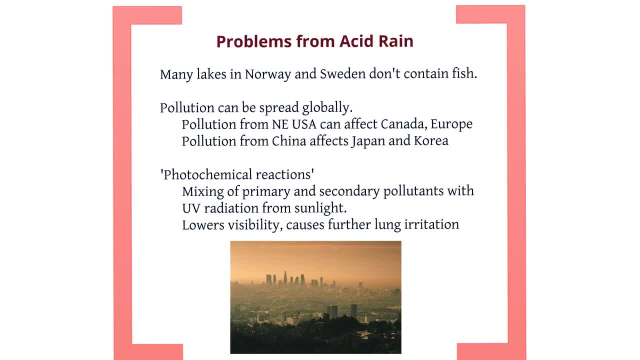 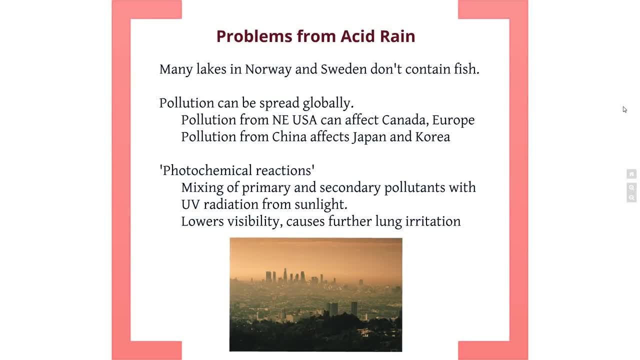 The mixing of primary and secondary pollutants with UV radiation for sunlight. This is the main reason why smog appears. It lowers visibility and causes further lung irritation. That's the picture of a city. I'm not sure which city, but it's a city. 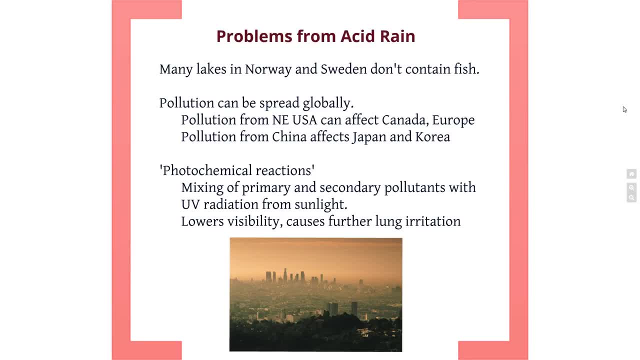 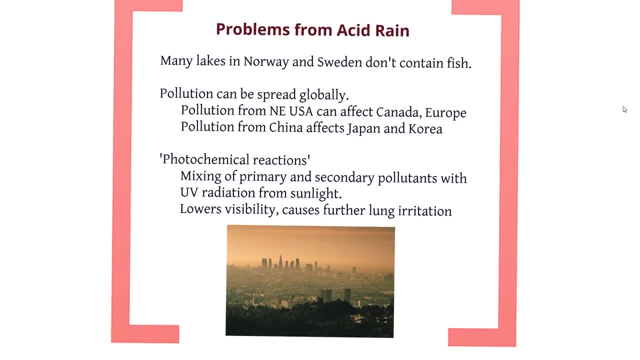 And most cities actually look like this now, where during the evenings you'll see a nice hazy smog covering the entire city. Not very pretty to look at, not very healthy to breathe in. Speaking of breathing in, they cause respiratory problems. 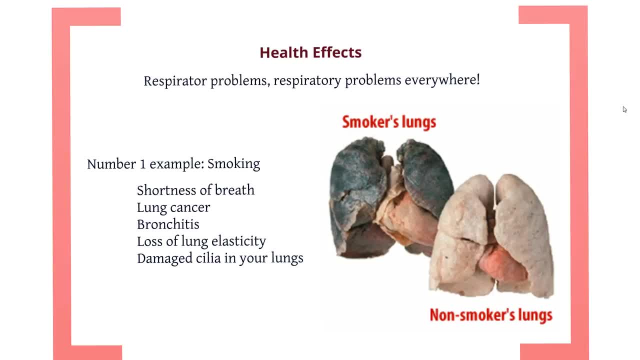 Respiratory problems everywhere. So the number one example that I can pull out is basically smoking. Prolonged exposure to any kind of air pollutants cause similar problems with smoking, but smoking is just a really concentrated form of that. It can cause shortness. 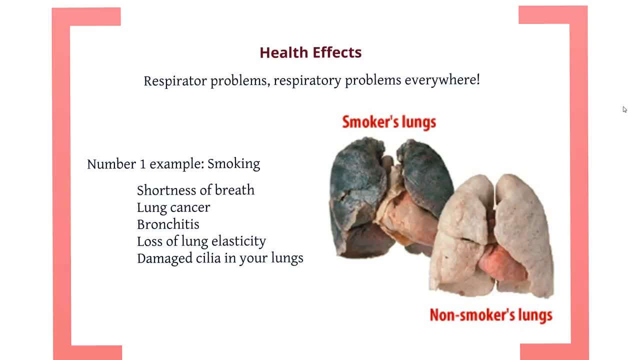 It can cause shortness of breath, lung cancer, bronchitis, loss of lung elasticity and damage to the cilia in your lungs, Not to mention it's not very pretty Moving on. so what can we do about it? 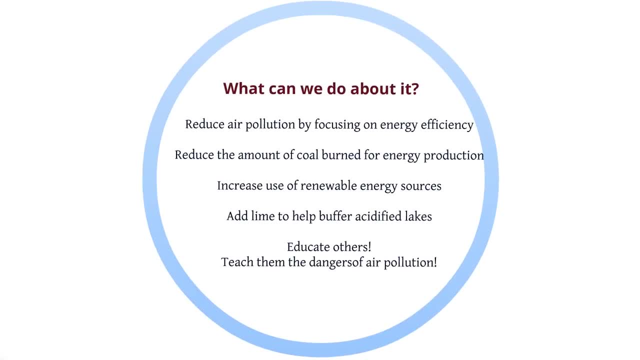 Well, first of all, you can reduce air pollution by focusing on energy efficiency. Burning less of it and being able to get more energy out of whatever you're burning is always better. Next, you can reduce the amount of coal burned for energy production. 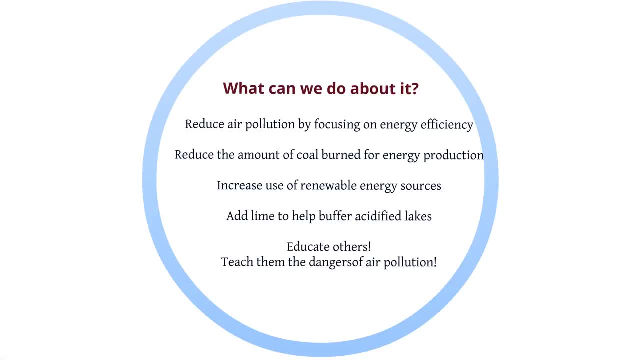 Focus on some other stuff like renewable energy sources. You can also add lime to help buffer acidified lakes. While it may not help lakes that have absolutely no life in them anymore, you can place lime into lakes to help buffer it a little bit, while they still do contain life. 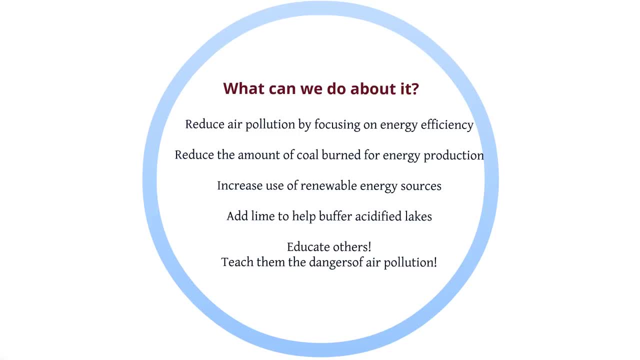 And finally, the most important thing is really to just educate others and teach them the dangers of air pollution so that they are more aware of what they are doing and they can help spread it to everyone else around them. Anyways, that was a quick environmental science overview of air pollution. Thank you for watching. I'll see you next time. See you next time.